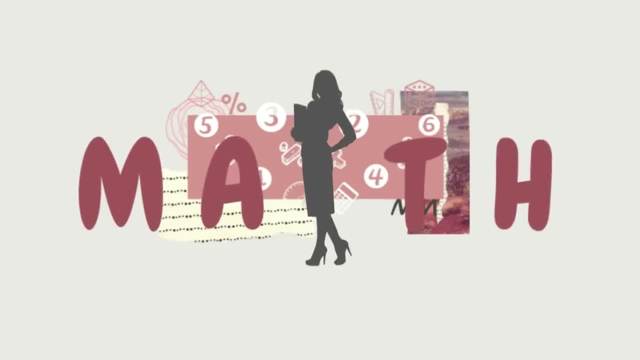 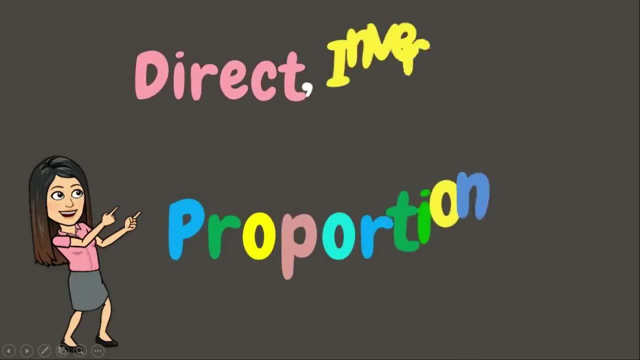 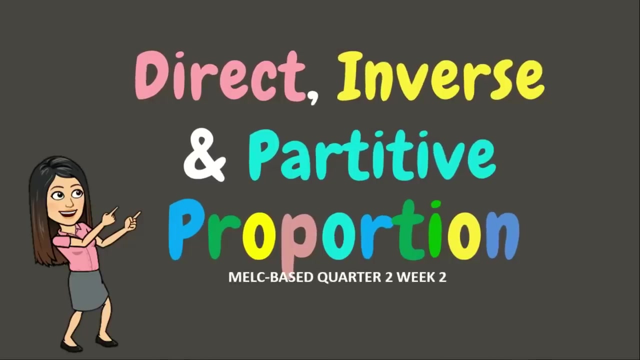 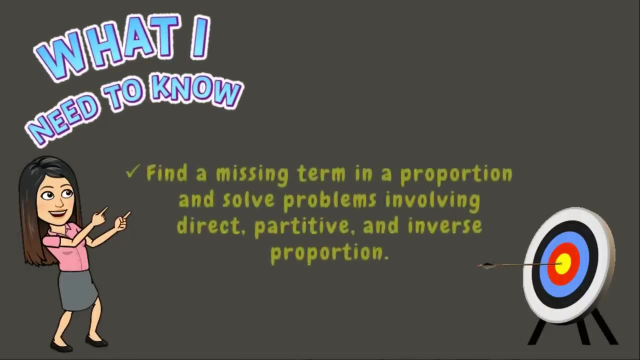 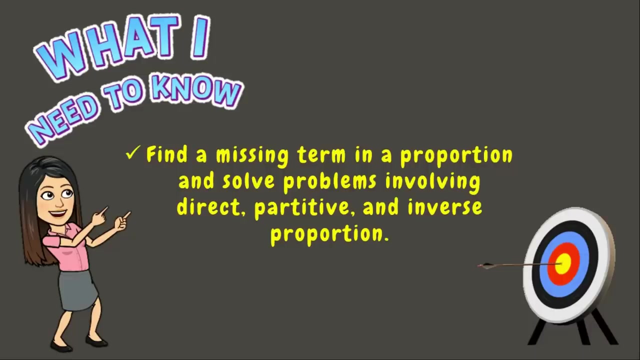 Direct, Inverse and Partitive Proportion. Great day, students. Welcome back to my classroom For today's lesson. you will learn how to find a missing term in a proportion and solve problems involving direct, partitive and inverse proportion. 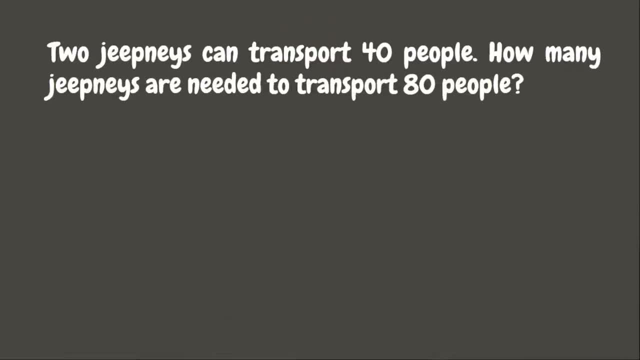 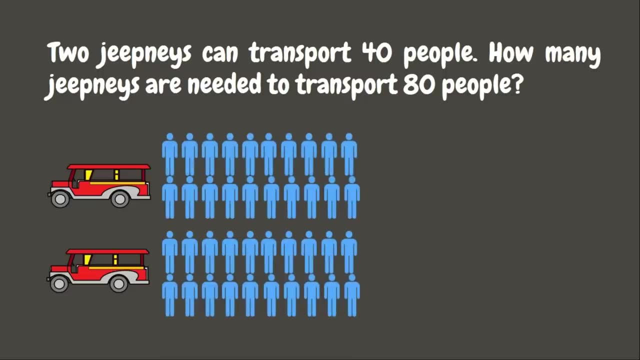 Let's begin. Let's try this first example. Two jeepneys can transport 40 people. Now how many jeepneys are needed to transport 80 people? Hmm, We can say from the given situation that the more people there is, the more jeepneys we need. 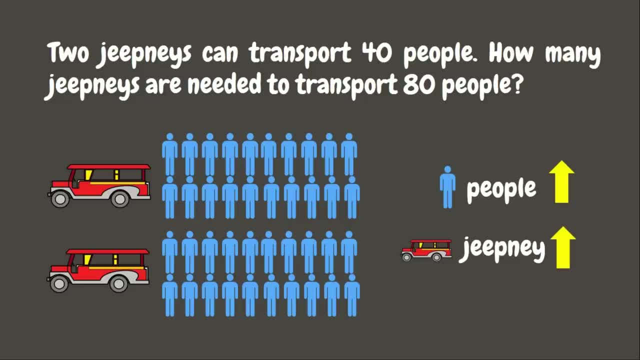 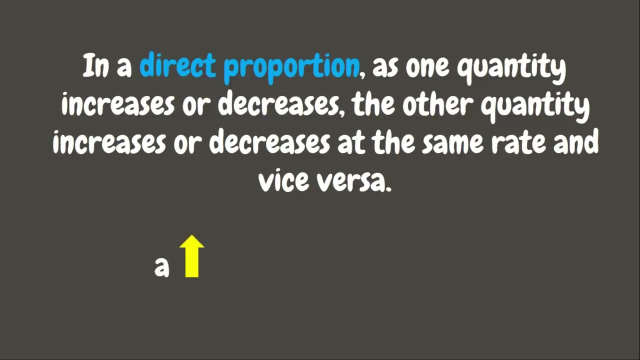 It means that when the number of people increases, the number of jeepneys should increase as well. This is an example of direct proportion. But what is a direct proportion? Hmm, In a direct proportion, as one quantity increases, the number of jeepneys decreases. 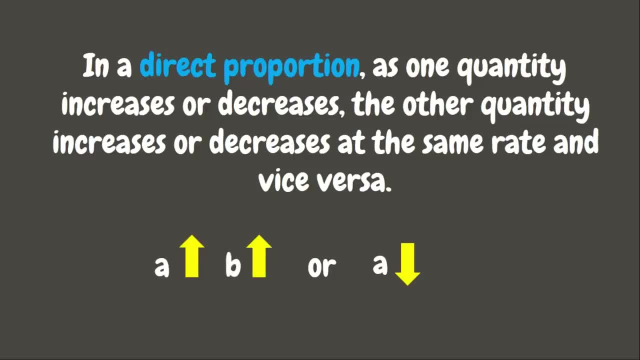 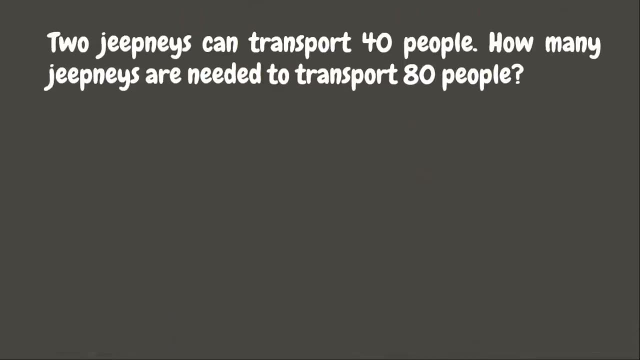 The other quantity increases or decreases as well at the same rate, and vice versa. Now let's go back to our problem. In solving a direct proportion problem, the first step is to identify the quantities used in the problem. Here we have the number of jeepneys. 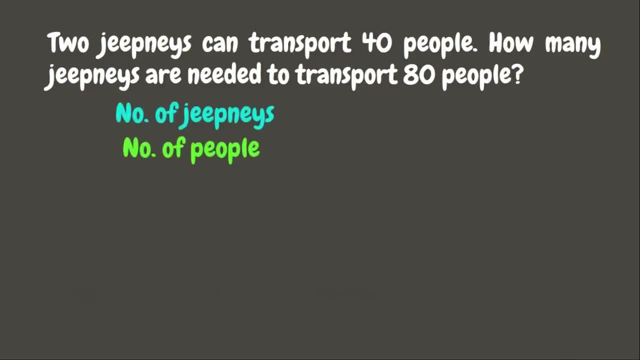 and the number of people. Now let's make a table. It is given that for every two jeepneys we can transport 40 people, And for every 80 people we are still looking for it. That's why let's put first letter N. 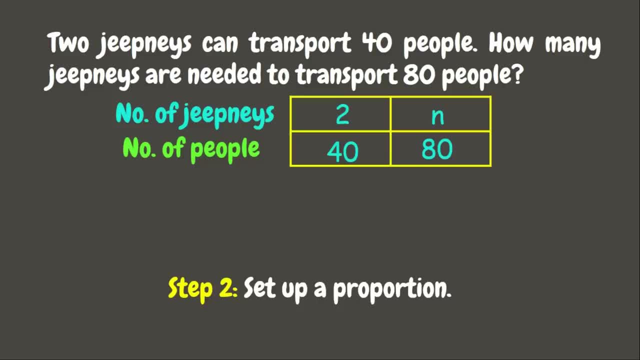 Now for the second step. let's set up a proportion. We have 2 over 40 people. We have 2 over 40 people. We have 2 over 40 people. This is equal to N over 80.. And for our third step. 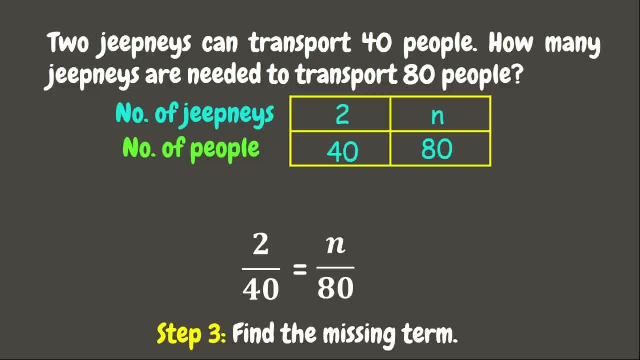 let's find the missing term, which is N. To find the missing term, we are going to use the cross multiplication method: 80 times 2 is 160.. 40 times N is 40N. But we are only going to write: 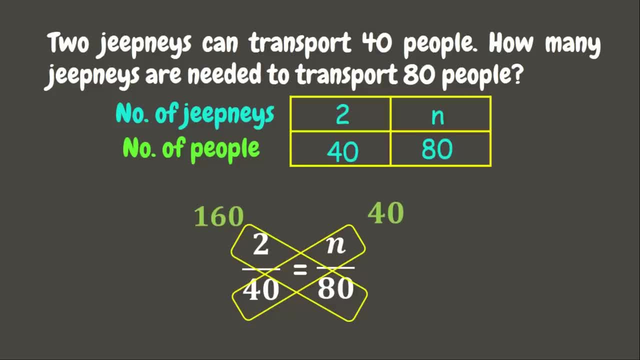 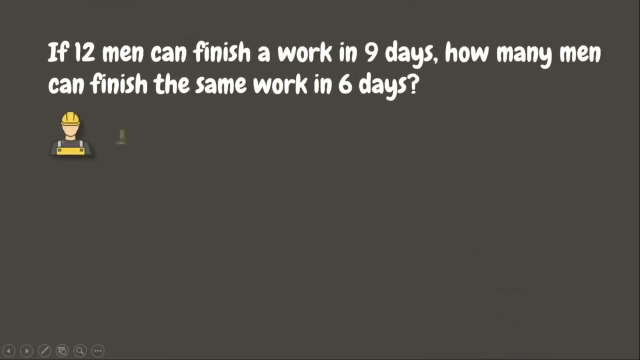 40, and the next step is: let's divide 160. divided by 40, it's for very good. that means there are four GPS that we need for 80 people. great job. now let's have our next problem: if 12 men can finish your work, 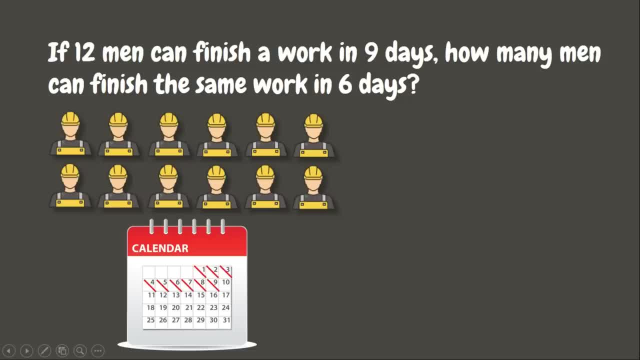 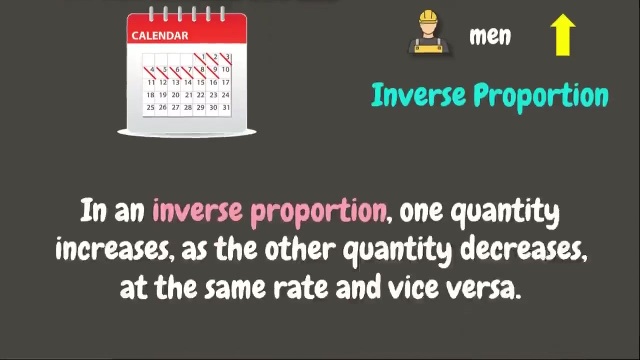 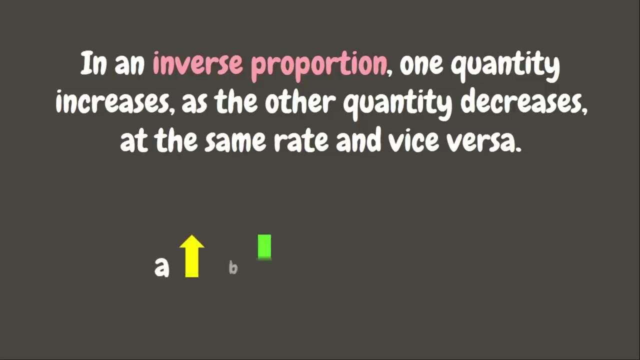 in nine days. how many men can finish the same work in six days? here, in the given situation, when the number of days decreases, the number of men should increase. this is an example of inverse proportion. now, what is an inverse proportion? in an inverse proportion, one quantity increases as the other quantity. 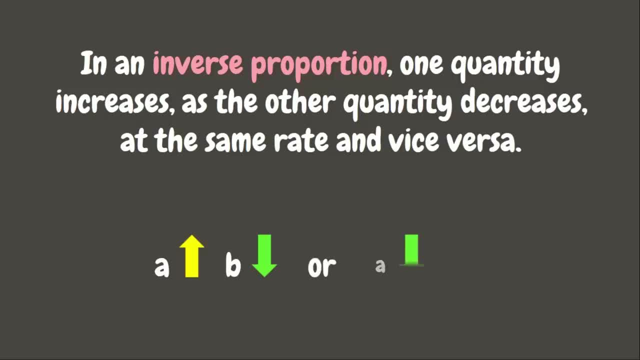 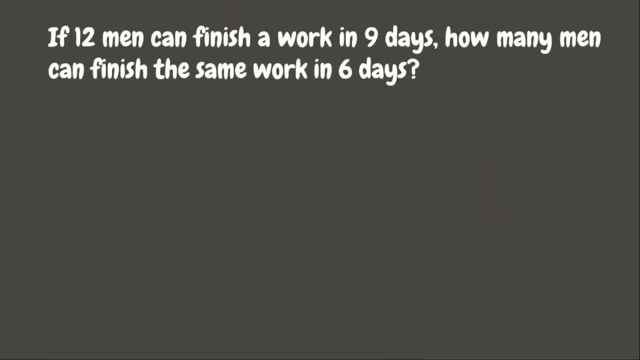 decreases at the same rate and vice versa. now let's go back to our problem. in solving in first proportion, the first step that we need to know is to identify the quantities used in the problem. here we have the number of men and the number of days it is given. the 12 men can finish a work in nine days. now, for six days we 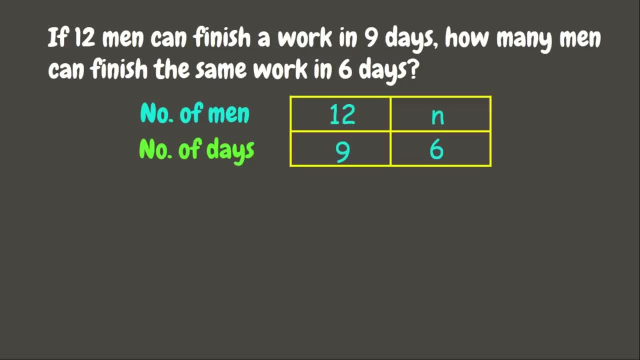 are still looking for it. that's why let's put N first. now the next step is to set up a proportion as indirect. by now. the next step is to set up a proportion as indirect by commonly seen as the number of men. in three months there now we do not know how many cases yet- we will create the feature that is, this name given number, and if you go in the page, the text is first. palette. now the next step is to set up a proportion as indirect, by interchanging the position of an. horizontally, let's interchanging the position of n't. horizontally, let's interchange the position of and. horizontally to the given number: 12. i'm gonna there, i'm gonna 열form. here you can see the saber다고 olsun, our favorite ver in the audience. 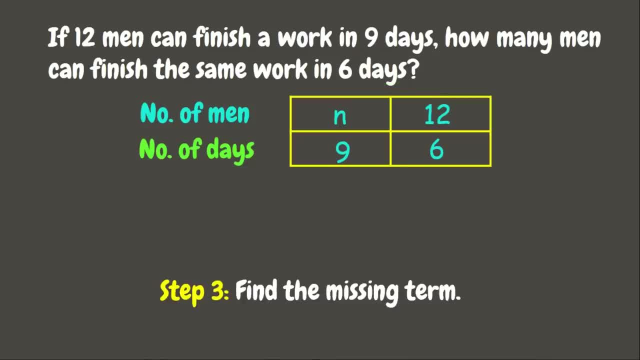 We are ready for our third step. Let's find the missing term. Our given proportion is: n over 9 equals 12 over 6.. Let's have cross multiplication 6 times n is 6n, but let's write 6 only. 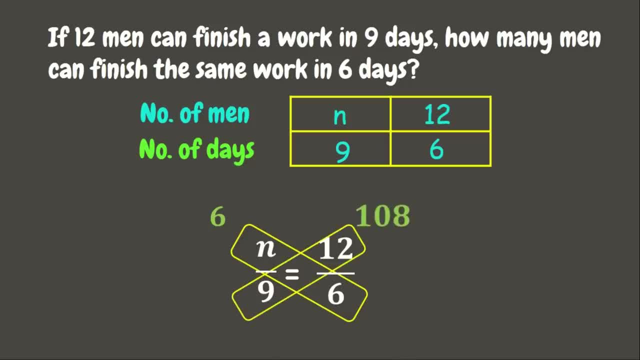 12 times 9 is 108.. Now the next step is to divide 108 by 6.. 108 divided by 6 is 18.. You are right. Therefore, n is equals to 18 men. This means that to finish the same work in six days. 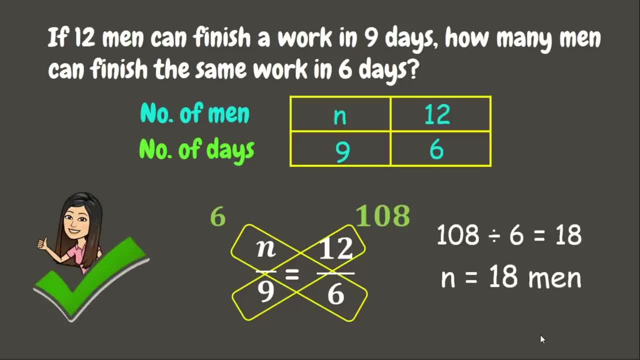 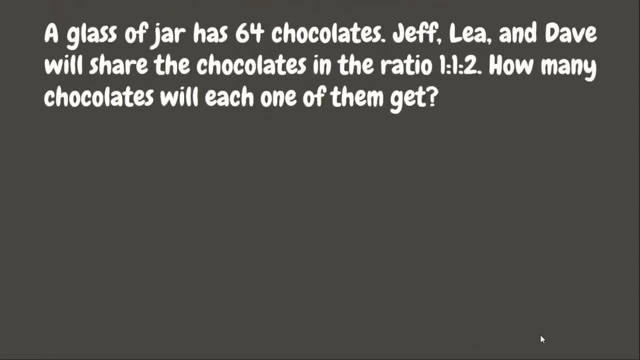 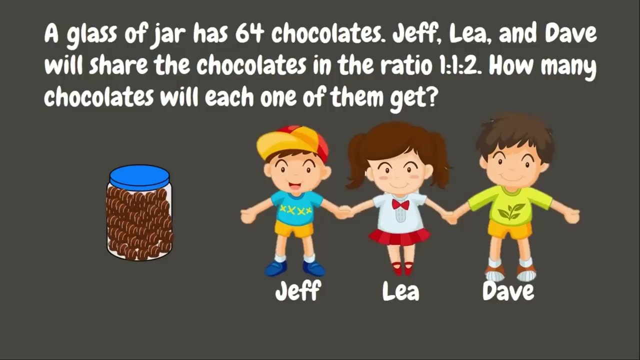 we need 18 men. Great job. Now let's go to our next and final problem. A glass of jar has 64 chocolates. Hmm, yummy. Jeff, Leia and Dave will share the chocolates in the ratio 1 is to 1 is to 2.. Now how many chocolates will each one of them get? 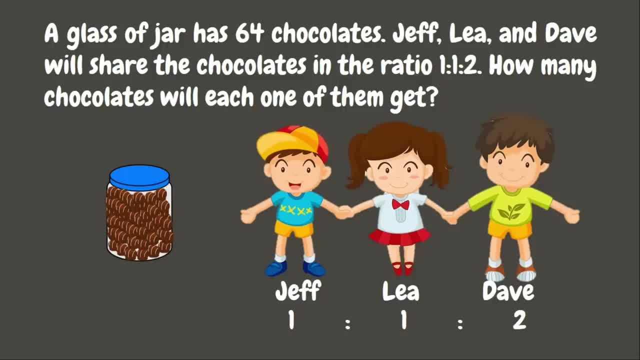 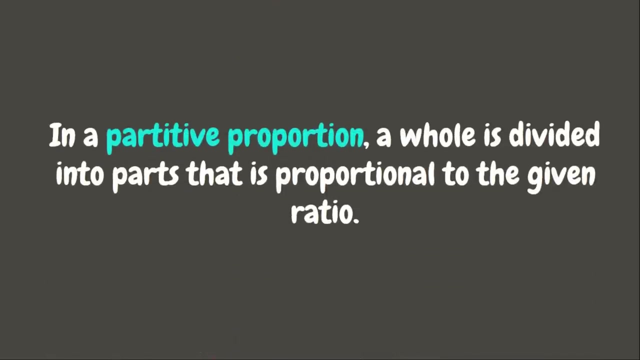 Here in the problem, we need to divide the 64 chocolates into Jeff, Leia and Dave. considering the given ratio, This is an example of a partitive proportion. Now, what is a partitive proportion? In a partitive proportion, a whole is divided into parts. that is proportional to the given. 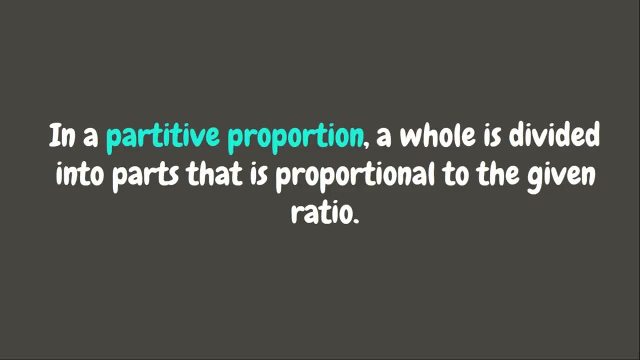 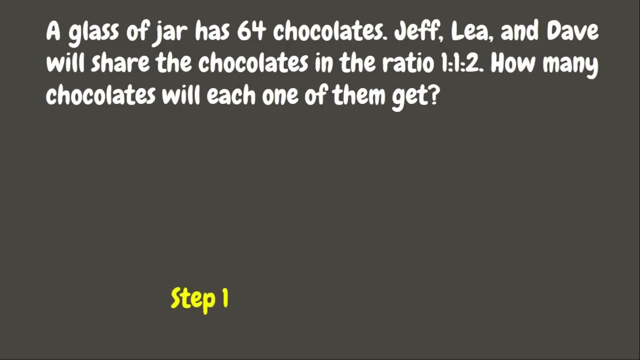 ratio. Now let's try to solve the problem. In solving partitive proportion, the first step is to find the sum of the ratio. Since the ratio is 1 is to 1, is to 2, let's add the numbers: 1 plus 1 plus 2 equals 4..